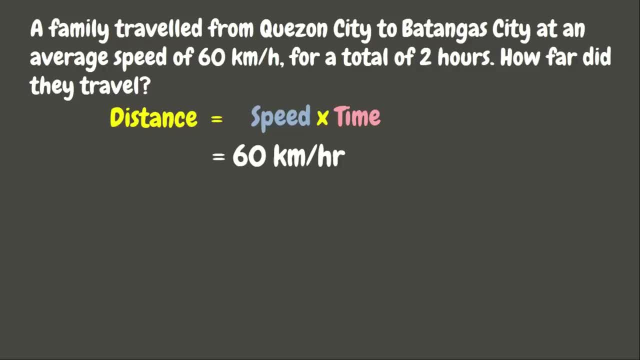 60 kilometers per hour, while the time is 2 hours. now let us solve. we have 60 times 2, which is great job. it is 120. now what could be our unit measurement here? we can already cancel the units of time, which is r, since r divided by r is 1, so we 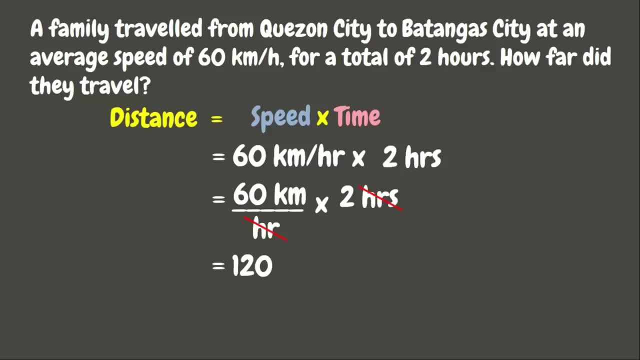 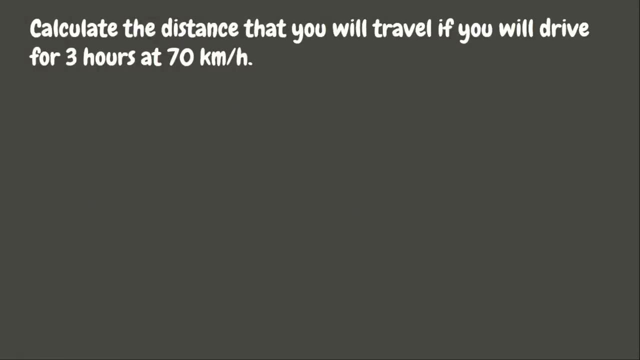 can simply cancel this out. and that leaves us the unit kilometers. therefore, they traveled 120 kilometers. now let's have another example. now let us calculate the distance that you will travel if you will drive for three hours at 70 kilometers per hour. again, to solve for the distance, we are going to multiply the speed and 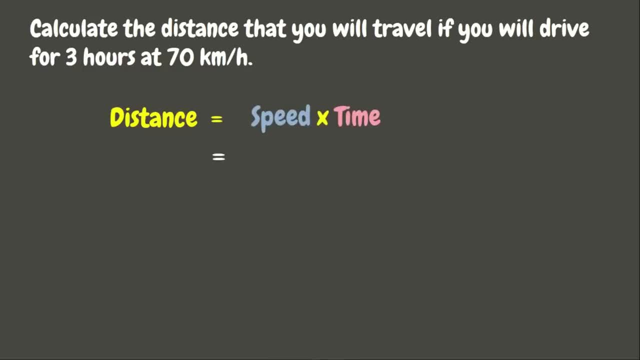 the time. here the speed is 70 kilometers per hour, while the time is 3 hours. now let us solve now: let's multiply 70 and 3 and that is wonderful: it's 210. now let's cancel the hours and now our unit would be kilometers. therefore, the distance will be 210 kilometers. 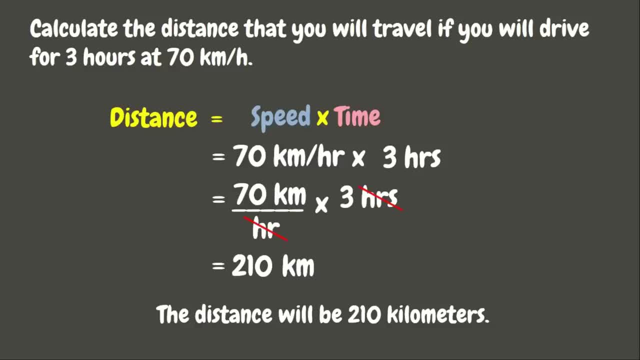 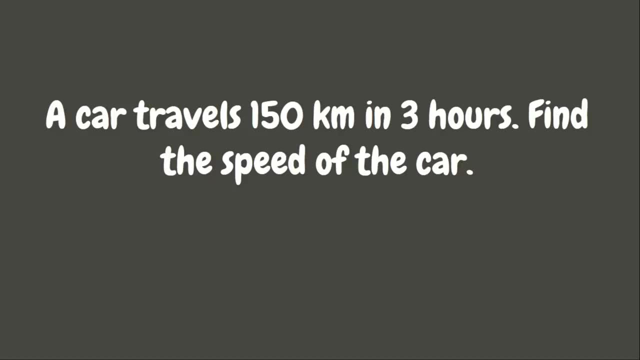 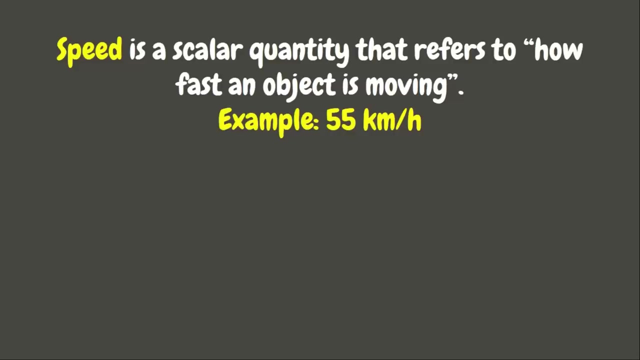 great job. now let's go to our next problem. a car travels 150 kilometers in three hours. find the speed of the car. this time we are looking for the speed. now, what is speed? speed is a scalar quantity that refers to how fast an object is moving. for example, we have 55 kilometers per hour. 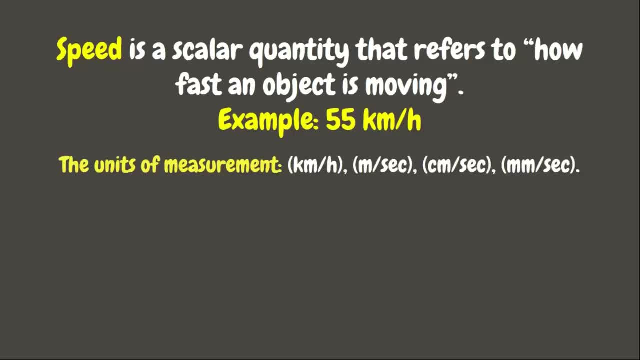 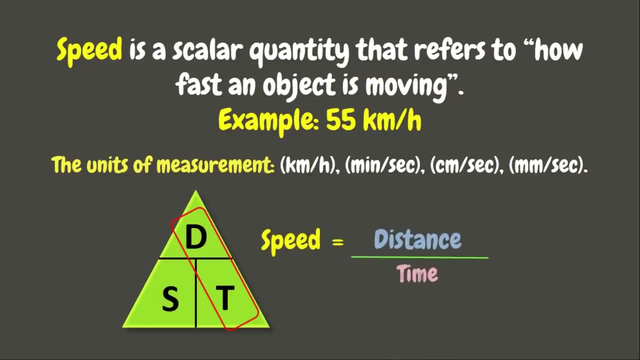 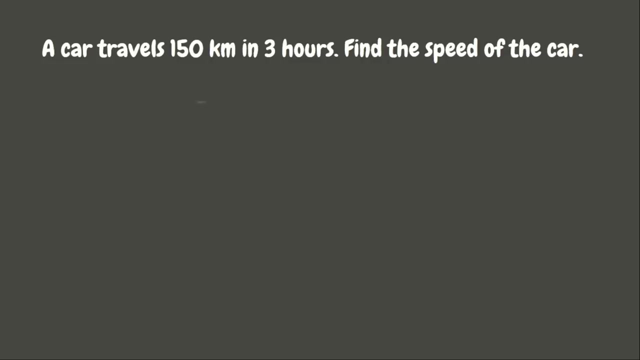 the units of measurement for speed are kilometer per hour, meter per second, centimeter per second or a millimeter per second. now, to solve for the speed, we just simply need to divide the distance by the time. now let's try to solve our problem again. to solve for the speed, we are just simply going to divide distance by the time here in our 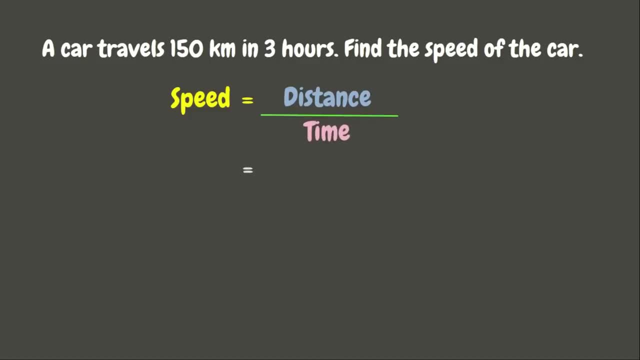 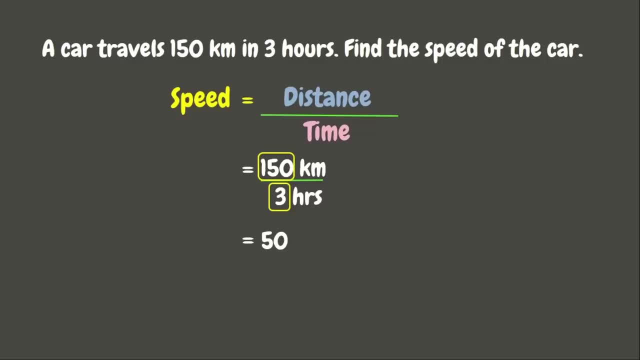 150 divided by 2. inch og isons km per hour. therefore the car travels 50 kilometers per hour. now let's have another example: find the speed when the distance is 280 kilometers and the time is 4 hours. again, to solve for the speed, we are going to divide the distance by the time, asking the находится at finish distance by the time. here in the Kurdish problem it would be the mileage time, getting the amount of miles per hour, and we're going to divide it by the time. 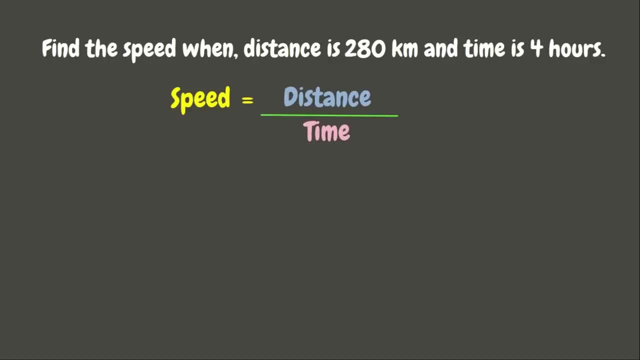 far from us now, in thekward conditions where the distances are rather short times per person and in large α see that only 50 kilometers per hour, we have going to suspended as dwa time here in a given problem. the distance is 280 kilometers and the time is 4 hours. now let us solve. 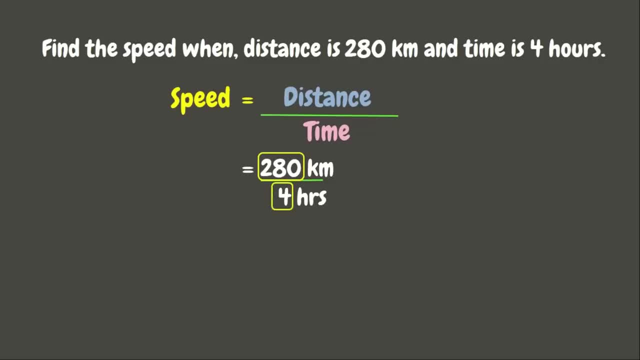 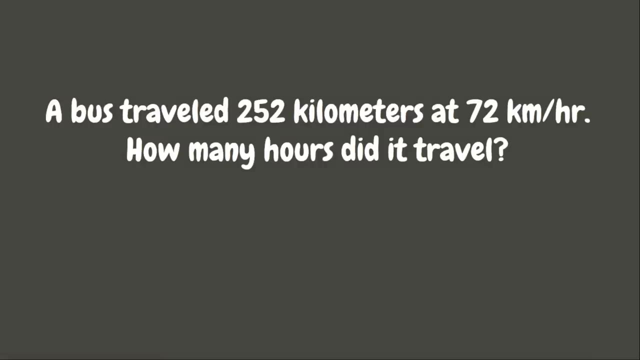 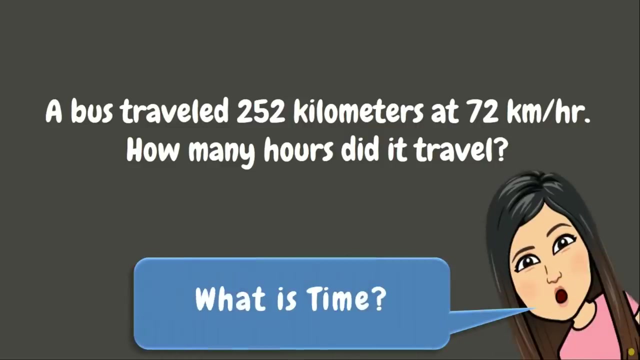 280 divided by 4 is wonderful. it is 70. so that would be 70 kilometers per hour. now let's go to our next problem. a bus traveled 252 kilometers at 72 kilometer per hour. now, how many hours did it travel? this time we are looking for the time, but what is time? 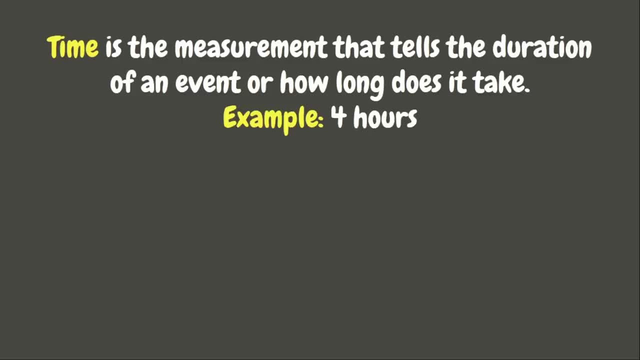 time is the measurement that tells the duration of an event or how long does it take. for example, we have 4 hours. the units of measurement for the time can be hour, minute or second. now to solve for the time, we are just simply going to divide the distance by the speed. 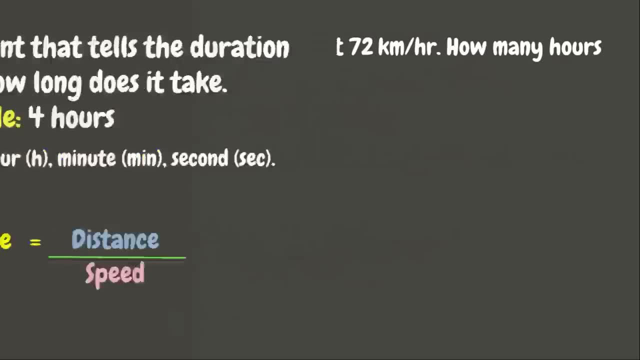 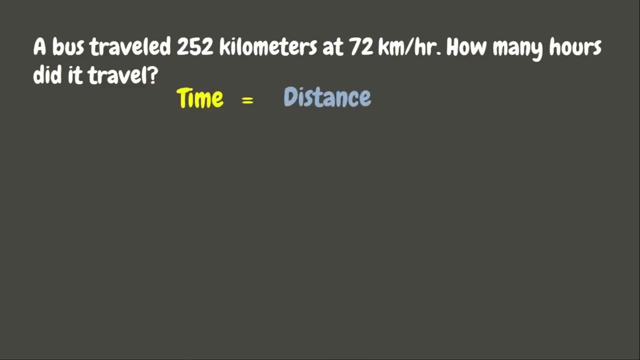 now let's go and solve our problem again to solve for the time, we are just simply going to divide distance by the speed. so here in our problem, the distance is wonderful, it's 252 kilometers and the speed is 72 kilometers per hour. now let us solve: 252 divided by 72 is awesome, it's 3.5 now, since we have two units of kilometer.